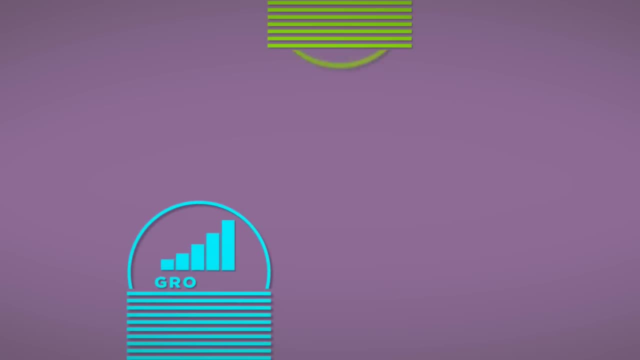 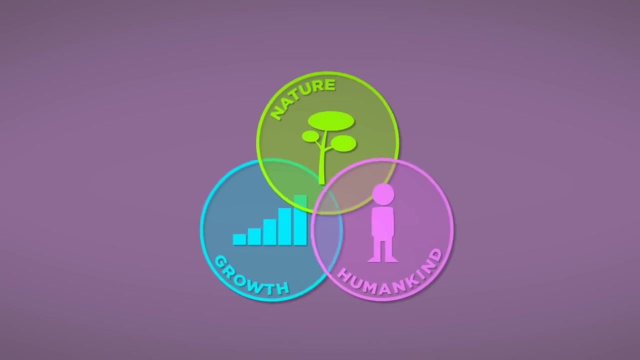 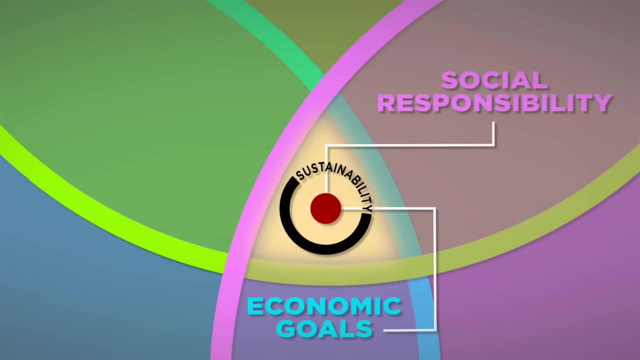 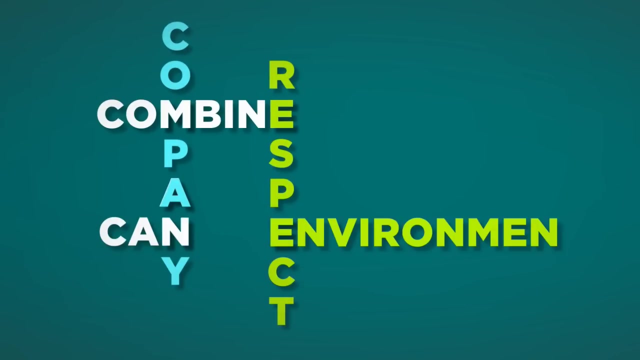 way. Sustainable development means that growth must be accomplished with respect for nature and humankind. And where is sustainability achieved? Right here, at the crossroads of economic goals, social responsibility and environmental protection. Now are you wondering whether a company can combine respect for the environment, social equity and commercial success? Well, the answer is yes. 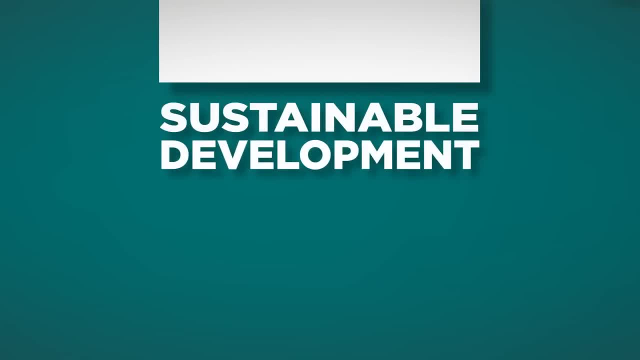 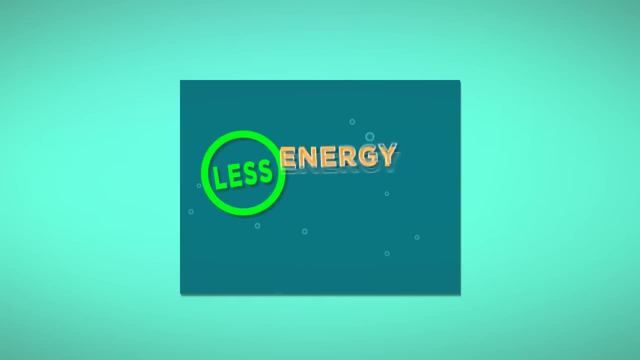 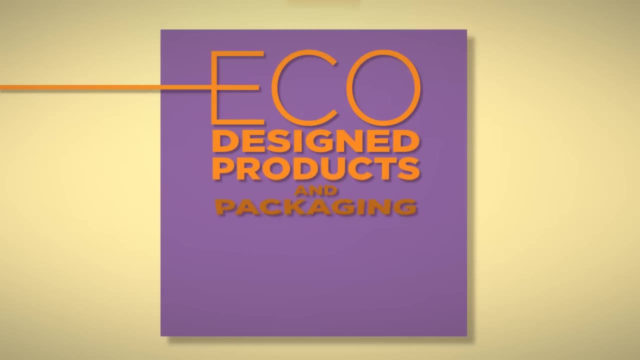 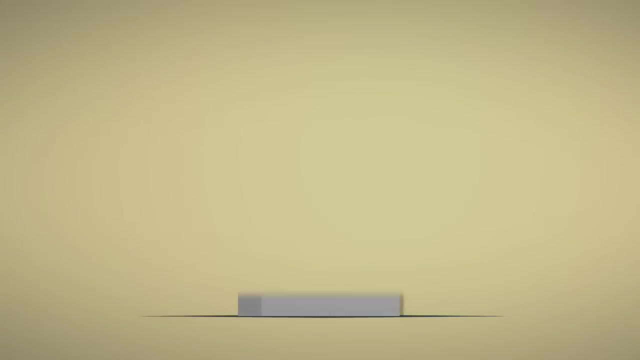 Not only that, but sustainable development creates value. Here's how Upgrading production tools to use less energy and water is good for the environment and for the pocketbook. Offering eco-designed products and packaging that use just what's necessary saves materials and reduces shipping costs. Paying attention to employees, improving their quality of life at work. 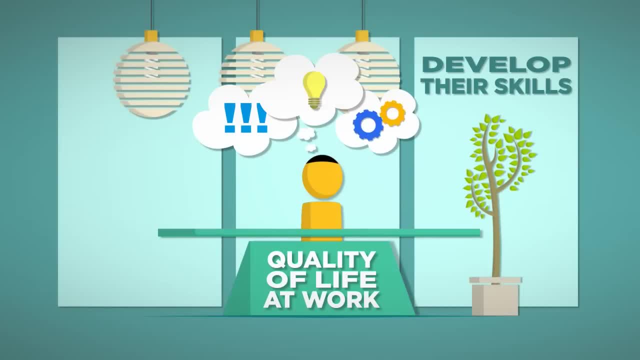 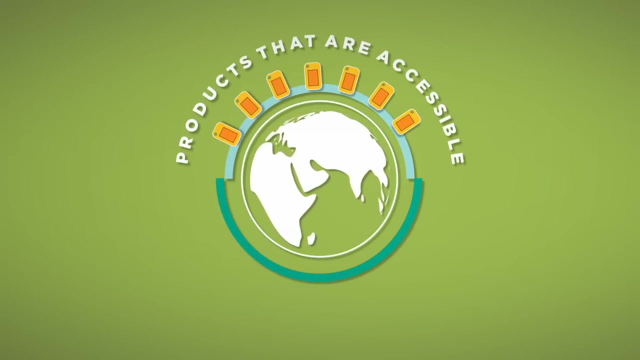 and helping them develop their skills all serve to strengthen their engagement, And stronger employee engagement means better overall performance, Creating products that are accessible to the world, Upgrading production tools to use less energy and water is good for the world's poorest populations, means opening new markets, the ones whose populations are going to. 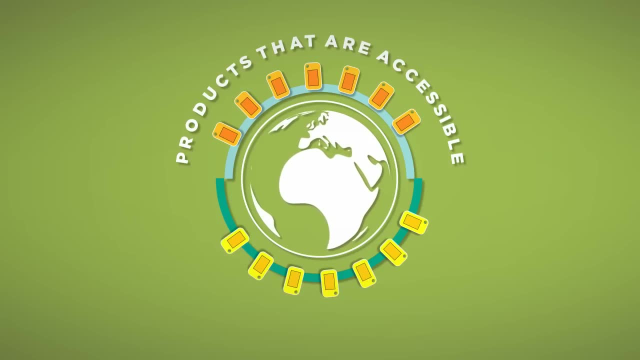 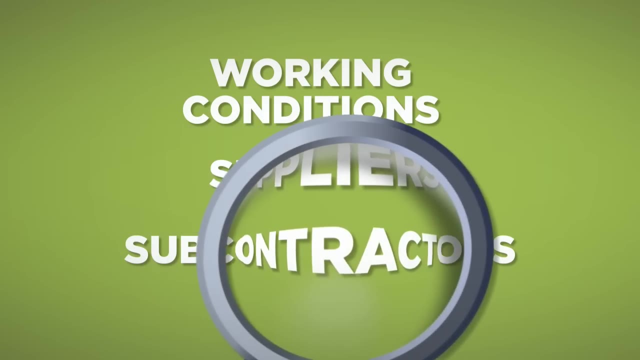 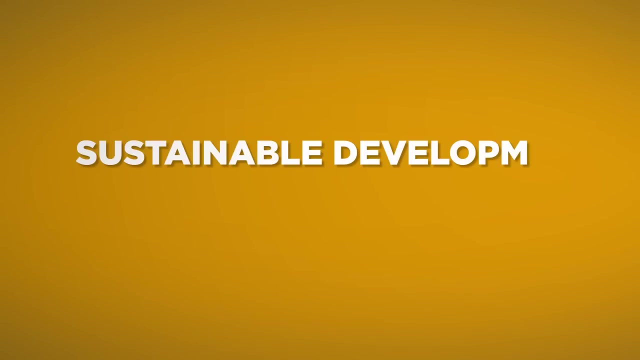 grow the fastest between now and 2050.. Monitoring the working conditions offered by suppliers and subcontractors means minimizing risks that could damage the company's image. As you can see, sustainable development affects just about everything. More and more companies today understand that they are the ones who are going to be the ones who are going to be the ones who are. 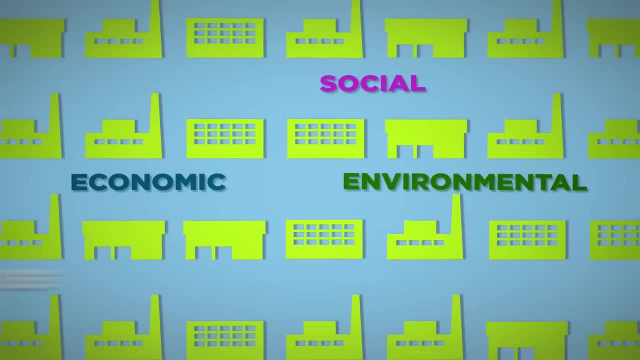 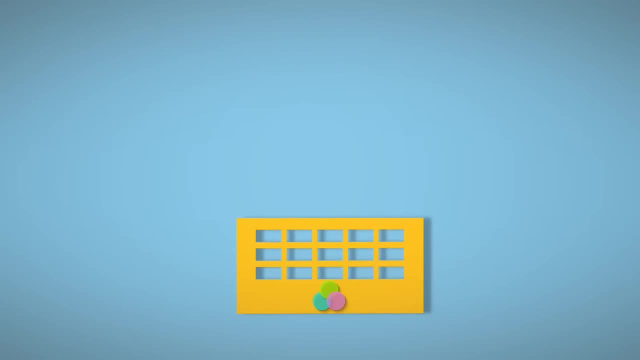 going to make a difference. They have important economic, social and environmental responsibilities and are committed to making a difference. The ones that seize this opportunity to create value will find that their success is, in a word, sustainable.